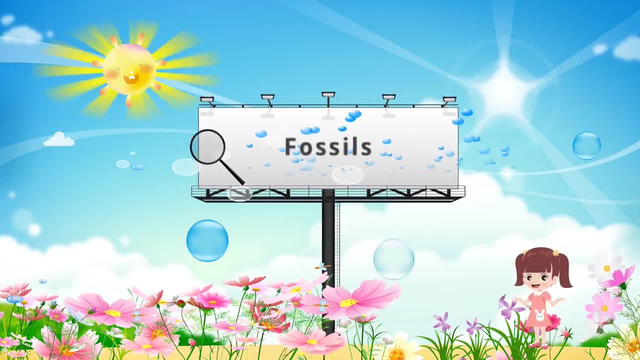 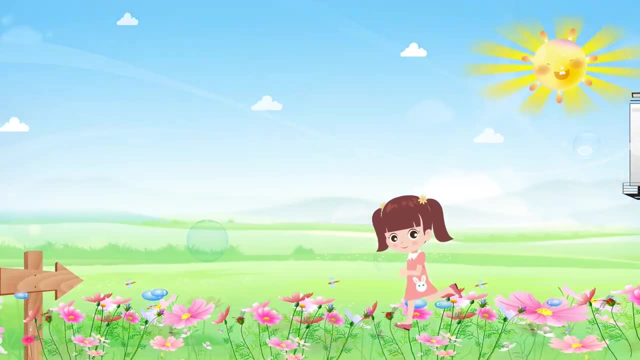 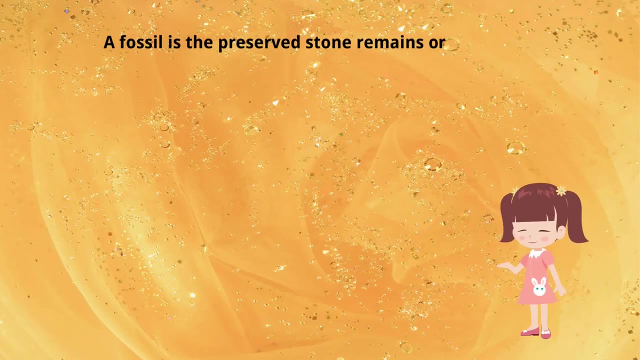 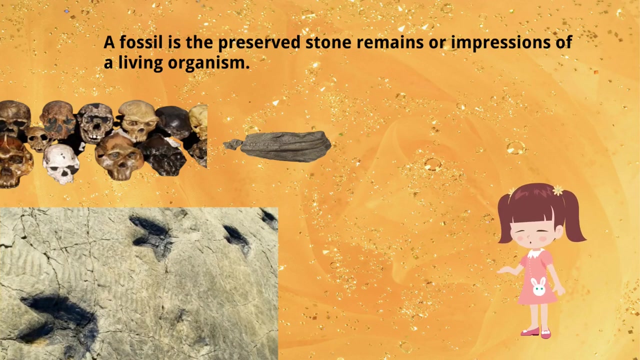 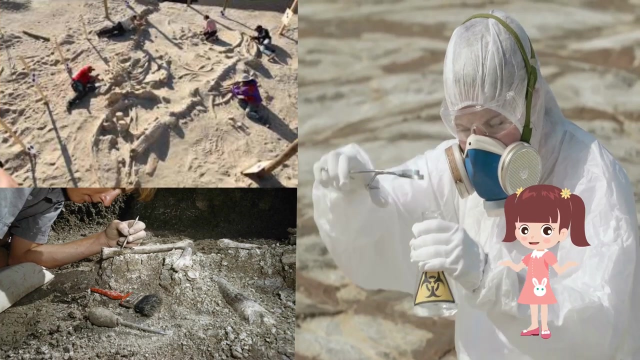 Hello friends, hope you are all doing well. In this video we are going to talk about fossils. A fossil is a preserved stone, remains or impression of a living organism such as a plant, animal, microbe or insect. Studying fossils helps scientists to learn about the history of life on. 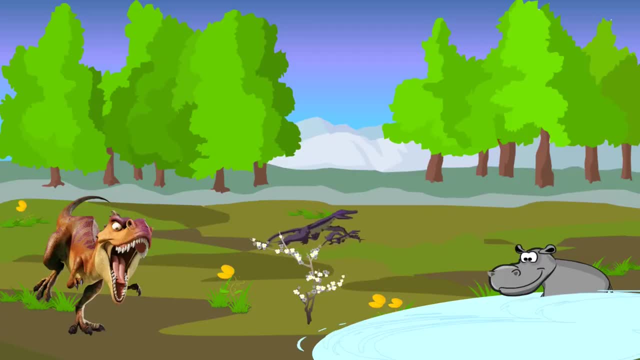 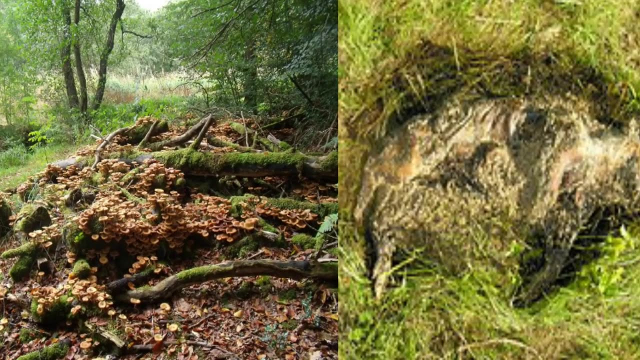 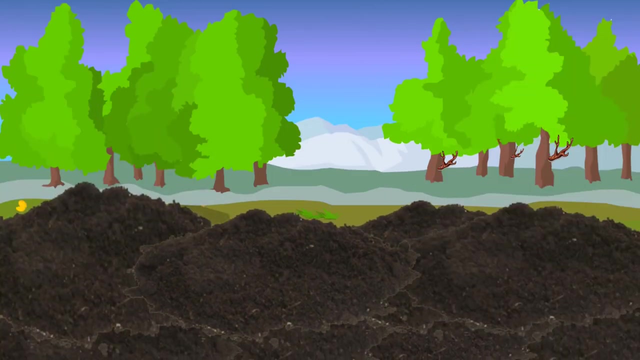 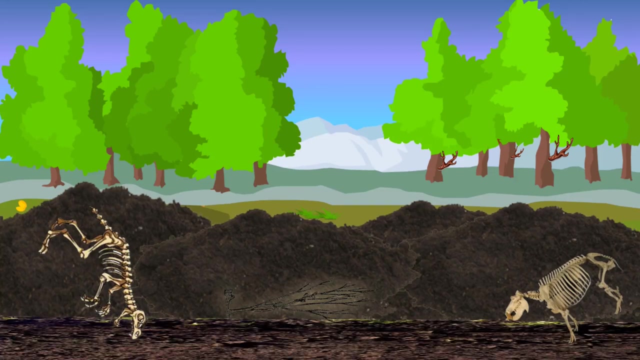 earth. Usually, the bodies of dead animals and other living things are completely destroyed, But sometimes they die in a watery environment and buried in waste that stop their decay. Soft tissues decompose, leaving the hard bones or shells behind. Over time, sediments build over the top and turn them into fossils. 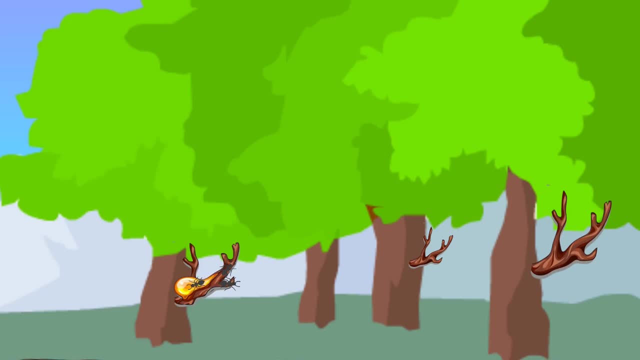 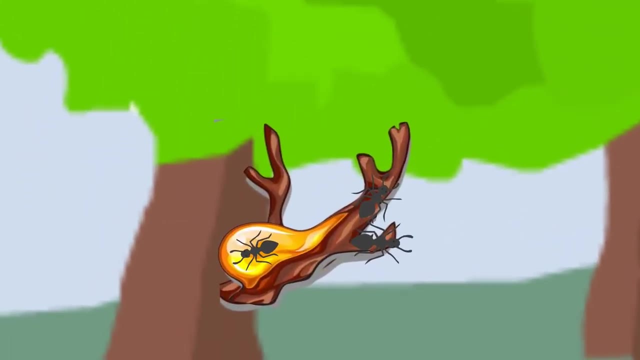 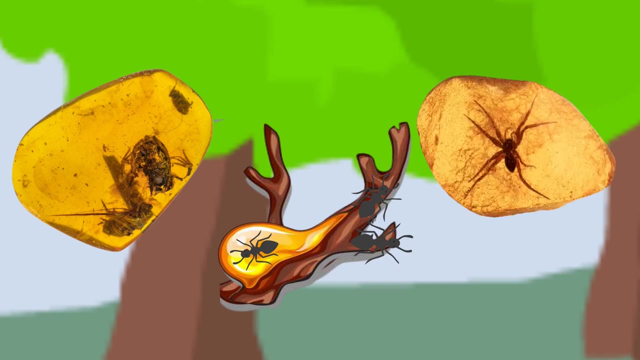 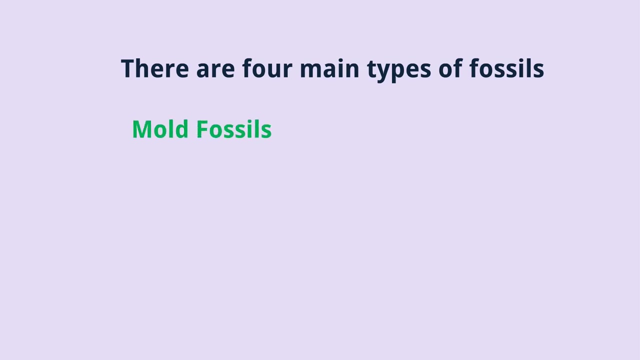 Insects can be trapped in the tree sap, which hardens and preserves the insects. The hardened tree sap is called amber. Amber preserves the fossils for millions of years. There are four main types of fossils: Mold Fossils, Cast Fossils, Trace Fossils and True Form Fossils. 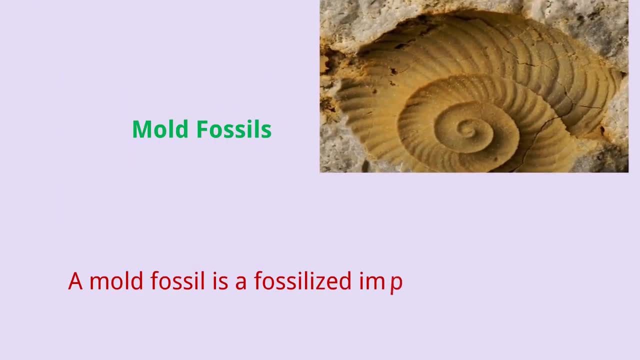 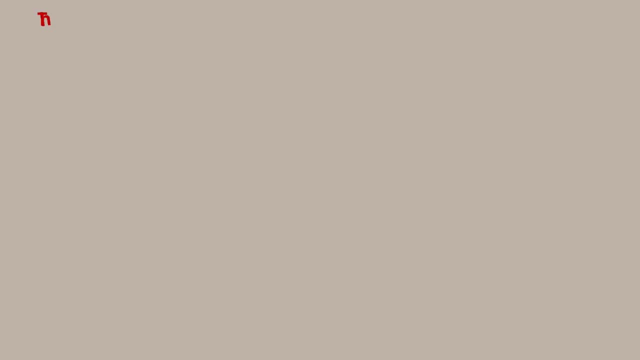 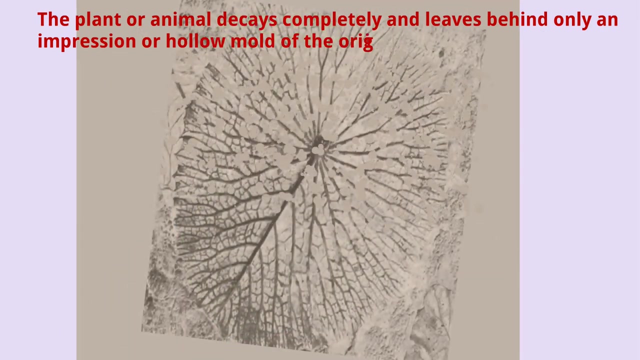 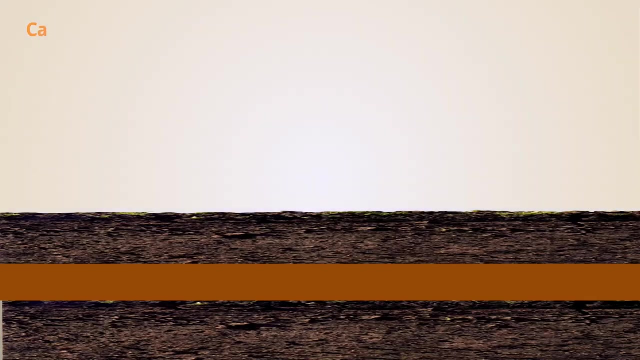 A mold fossil is a fossilized imprint made in sand or clay. The plant or animal decays completely and leaves behind only an impression or a hollow mold of the original organism. Cast fossils are one step ahead of mold fossils. Cast fossils are formed when a hollow mold is filled in with some sort of minerals.